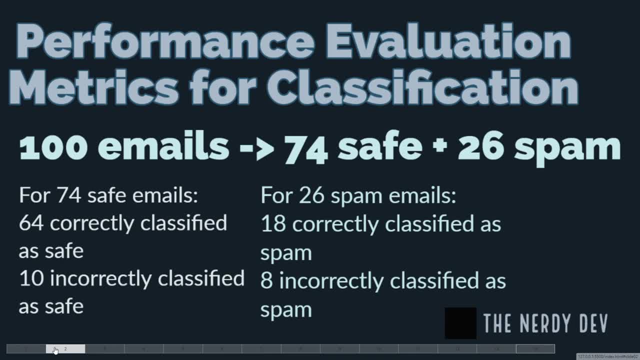 spam, that is spam emails. they are safe emails and say: 26 emails are your spam emails. now suppose we have a classifier model that was trained on the dataset and it correctly classified 64 out of 74 safe emails as safe and rest as spam from the remaining emails. out of 100, that is 26 spam emails. it. 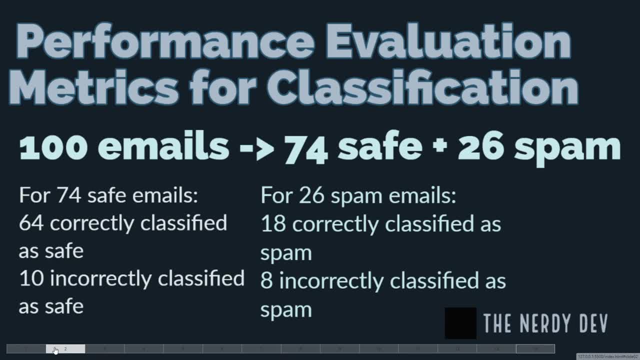 correctly classified 18 emails out of these as spam, but failed to classify the rest of the emails as spam spam. so how many incorrect classifications were made by our model for the safe emails that we were having in a collection of handed emails, 10 were incorrectly classified as safe and 8 were. 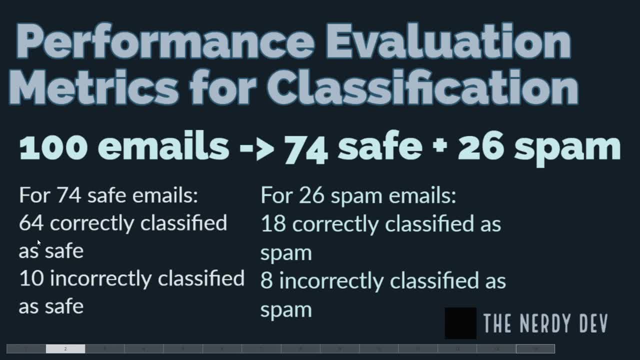 incorrectly classified as spam. so in all we have 18 misclassifications or 18 incorrect classifications, so it's clear that the model made 18 incorrect classifications. or you can see that our model made 18 errors, so you can see that the number of correct classifications is 82 and the number of 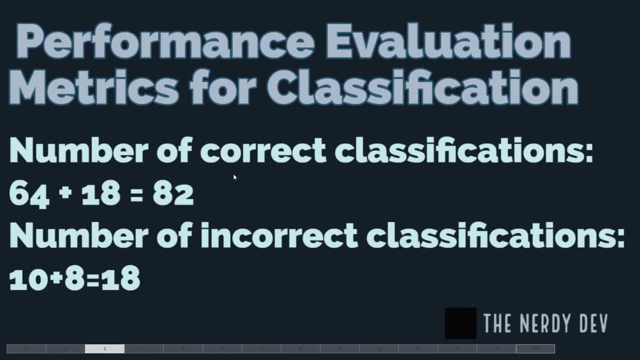 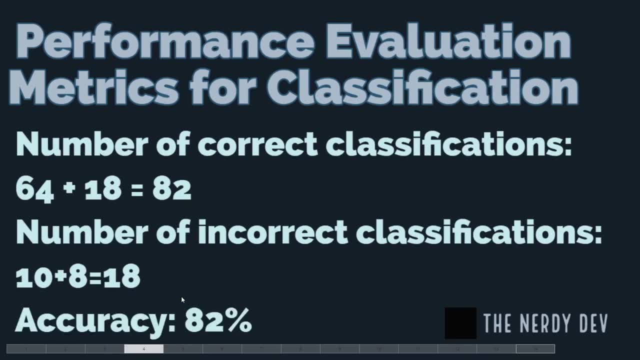 incorrect classifications is 18, so number of correct classifications is 82 and number of incorrect classifications is 18, so we can see the accuracy for our model comes out to be 82 percent. so now, before proceeding to other classification metric, let us first understand the problems. 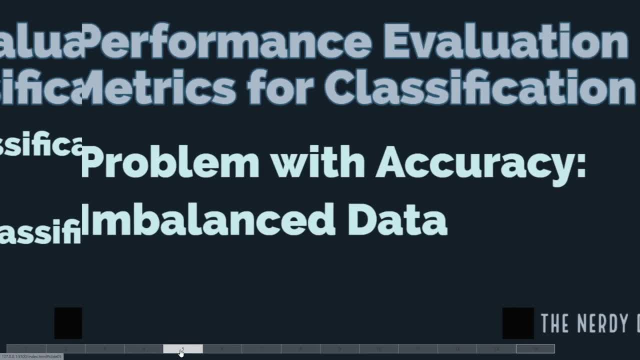 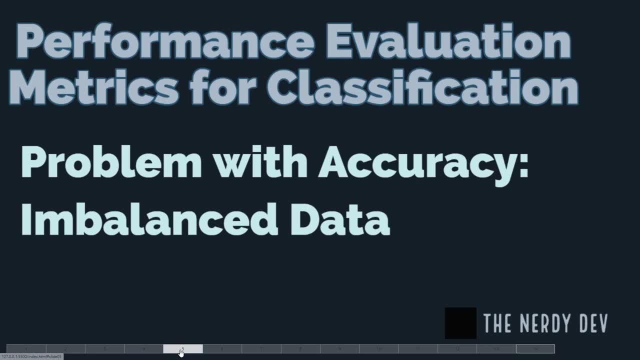 associated to this classification metric and that is imbalanced data. so suppose you have your test data set and in that we have 75 percent of our test data indicating that the email is not a spam, which is it indicates that email is a safe email, and 25 percent of the test. 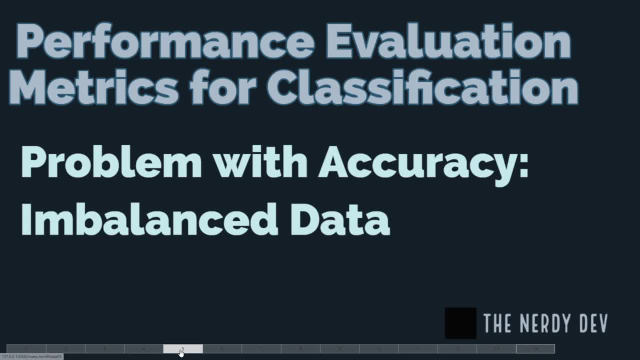 data. the very same test data indicate that the email is a spam. now, because of the problem, what will happen is that the model will give a false impression of high accuracy because, as you can see, that 75 percent of your data set is incorrect. so you can see that the model made 18 errors. 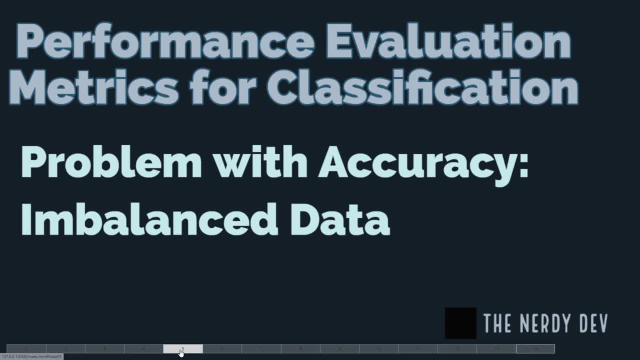 occupied with emails that are safe emails and only 25 percent are those that are in spam clause, thus giving an incorrect accuracy of 75 percent based on imbalanced data. so this means that accuracy is not a good performance metric for imbalanced data, so avoid using accuracy as a metric. 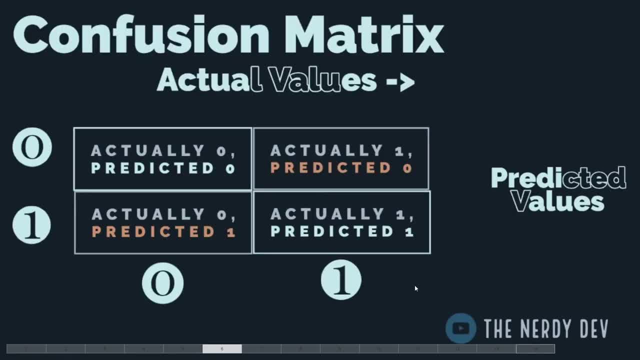 when we have imbalanced data in our data set. so now let us move to another concept here, which is called as the confusion matrix, and let us understand how it can help us. so, as a simple example you can see. so as a simple example, let us take a case of binary classification. that is, we have two classes, class zero and class one. 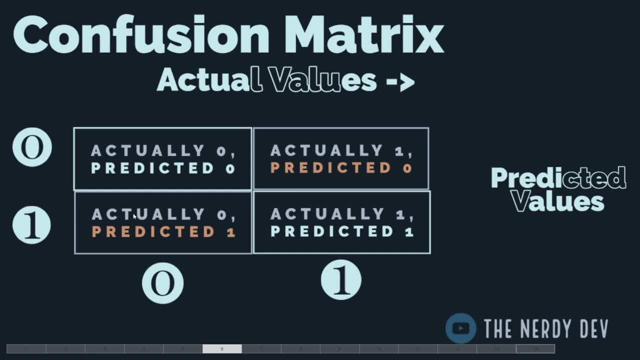 so, as you can see, we are having a two by two matrix with two rows and two columns. now the order of the matrix is two cross two, because in binary classification we will deal with two classes. so suppose we have a test data set with k data points where, for each such data, 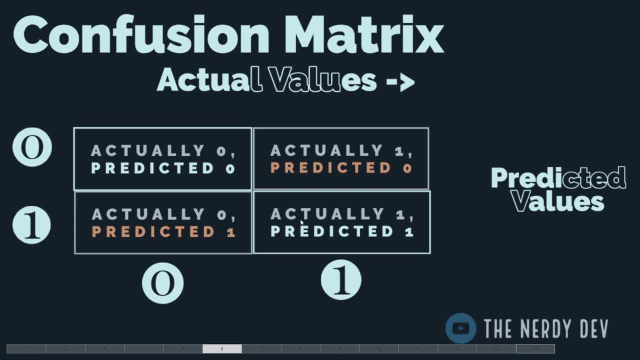 point, we have the actual class label, that is, the actual value provided by the data set, because you know, we are dealing with supervised learning in case of classification and, let us say, for each data point, we also have the predicted value represented by y cap. so you can see that there are only four possibilities. that is the first possibilities: actual label. 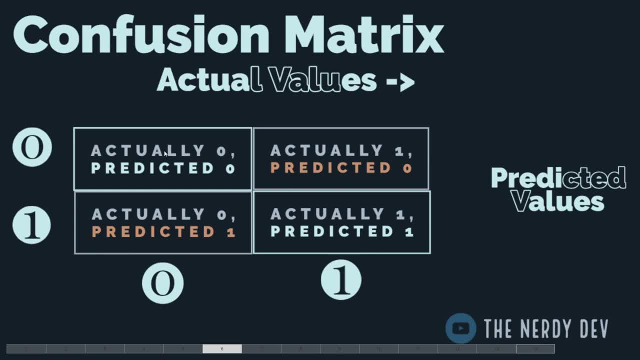 is zero, which is represented by the first cell of your confusion. matrix and predicted value. zero, which corresponds to the data set, value of the data set, which is the actual value of the data set. to a correct classification Now case 2, with actual value as one and the. 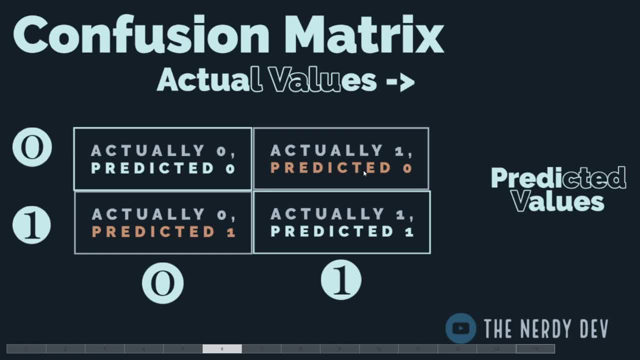 predicted value is 0, which corresponds to an incorrect classification. at this with red shade. Now case 3: actual label is zero, predicted value is one which corresponds to an incorrect classification. and the case 4 is: actual label is one. predicted value is one which corresponds to a correct. 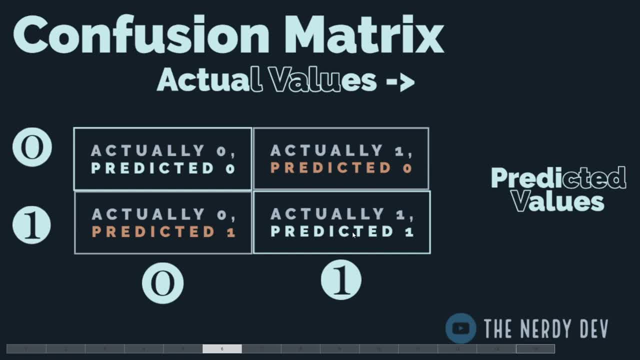 classification. Now this concept can be easily extended to a Multiclass classifications where you may have n such classes and then it will be a n cross n confusion matrix. so if the number of correct classifications, that is, the elements that are there along the diagonal of your confusion matrix, on the principal diagonal of your confusion matrix, such classifications. 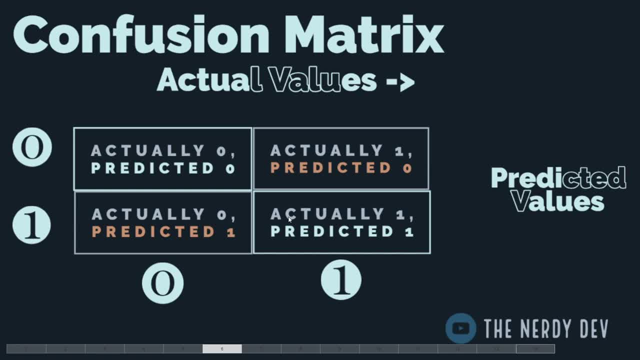 are on a higher side, then you can conclude that your model is doing reasonably well and it has a decent statistical power of prediction. on the other hand, if number of correct classifications are on a lower side, that means your model is a poor performing model and it didn't learn well in its training process. now remember that i said in the previous videos. 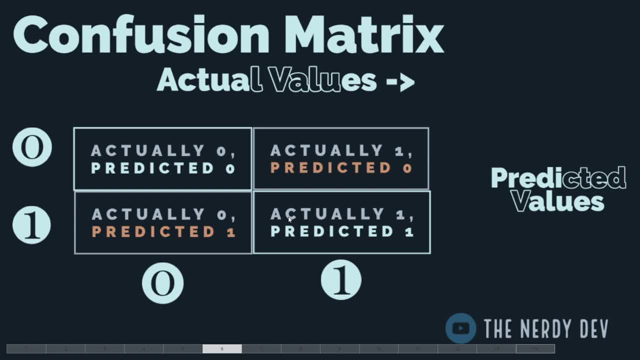 that no model is a perfect model. each and every model will have some error element associated to it. this discussion simply boils down to one more result: that all the principal diagonal elements are on the lower side of your model and it has a decent statistical power of prediction. 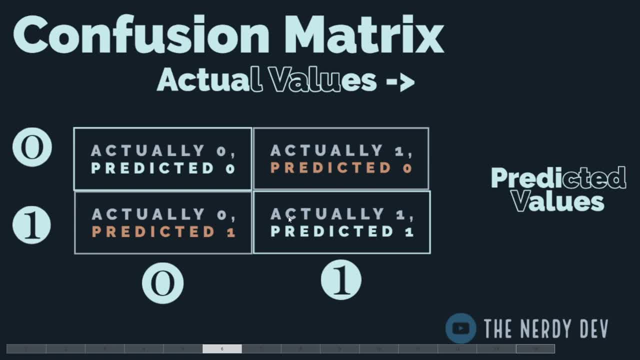 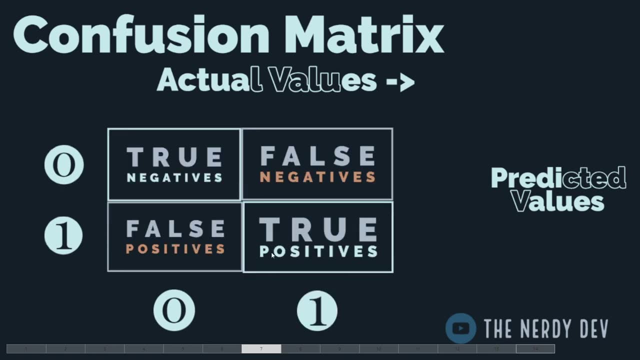 in case of a confusion. matrix should have high number of correct classifications in order to have an overall estimation of the statistical power of prediction of your model. so do take a note of this result. so now there is a term for each cell of the matrix, and let us discuss about. 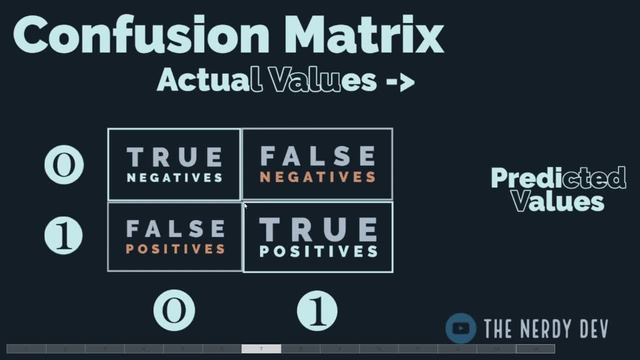 them now. so this cell represents a true negative, which means that the actual value was a zero. so the actual values are represented horizontally. so this zero and this one represents the actual value which is along the x-axis, or you can see, along the horizontal axis, and the predicted values are represented vertically, so predicted. 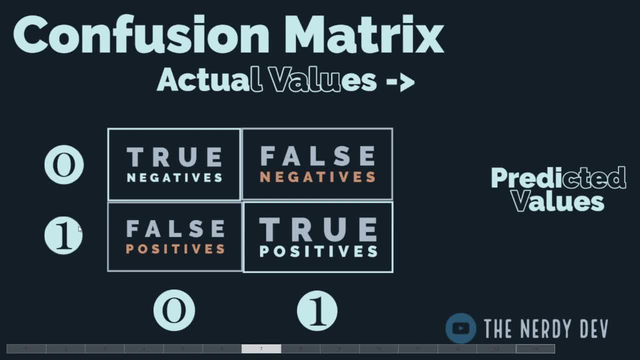 0 and predicted 1.. so the actual values are those values that serve as the labels in your data set, and the predicted values are those that are predicted by our model, and we are having only two values, 0 and 1. so there is a term for each cell of the matrix, and let us discuss about them. 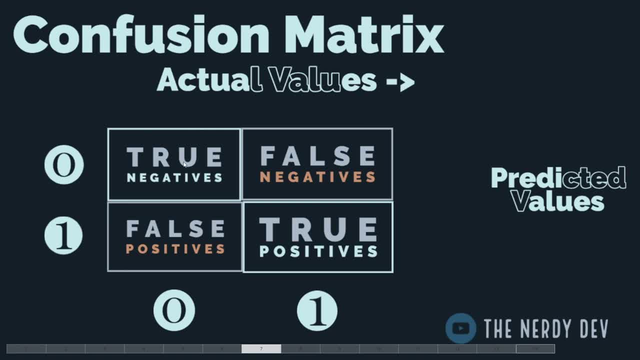 now, this cell, the very first cell, which is this one, represents a true negative, which means that the actual value was zero. so actual value which is represented by this zero where my cursor is currently sitting on, and the model correctly predicted it as a zero. so this is a true negative. 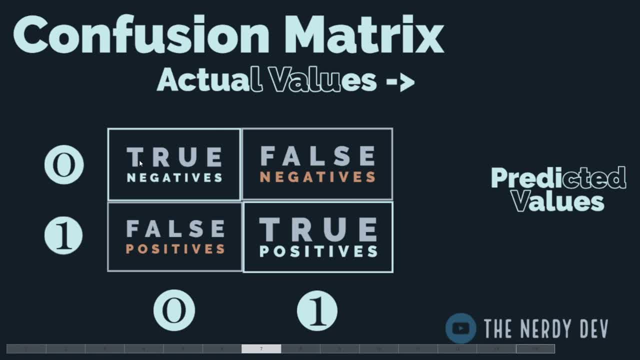 so actually it was a zero and the model correctly predicted it to be a zero. that means true negative. so we are seeing it as a negative because we consider here zero as the negative class and one as the positive class. then this cell represents the false negative, which is this one, which means: 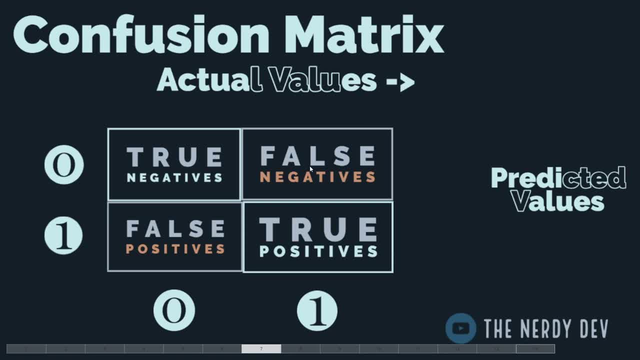 the actual value was a. one was a positive class, but the model incorrectly classified it as zero. okay, so this cell then. this cell represents false, negative means. actual value was one, so as you can see from the diagram, but the model incorrectly predicted it as zero. that means it incorrectly classified points that were actually one as zero. then, coming to the 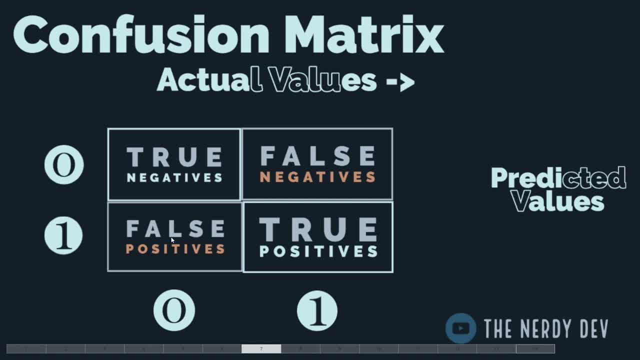 third cell, which is this one. it represents false positives, means that the actual value was a zero, but the model incorrectly classified it to be a positive class or to be a one, which means a false positive. so the model falsely predicted it to be a one, but actually it was a zero. moving on to the 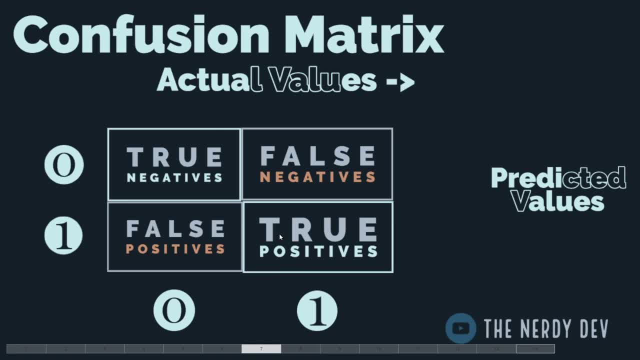 last cell. this represents true positive, and what it means is that the actual value was a positive class, or it was one and the model correctly predicted it to be a one, and hence the term true positive for it. so now let us discuss about some terminologies. now, if we sum up the elements along the two columns, for the case of binary classification, 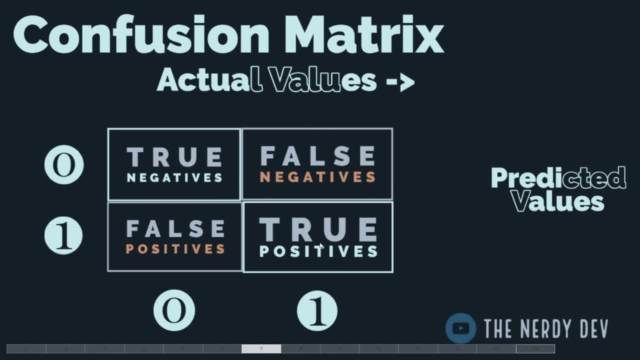 we have p as the number of actual positives, which is false negatives plus true positives. you can use small p and the number of actual negatives can be denoted using small n, which is true negatives plus false positives. so now let us discuss about some very important terms pertaining to the 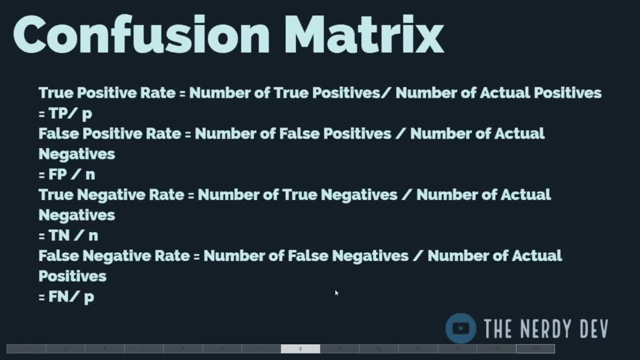 confusion matrix. so we have the true positive rate, which denotes the number of true positives upon the number of actual positives, which is tp divided by p. then we have false positive rate, which is fp divided by n. then we have the true negative rate, which is the number of true negatives. 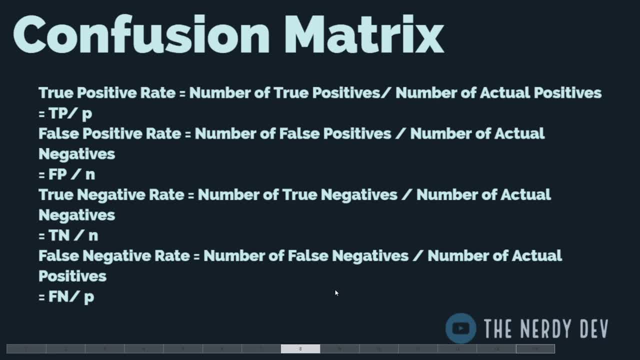 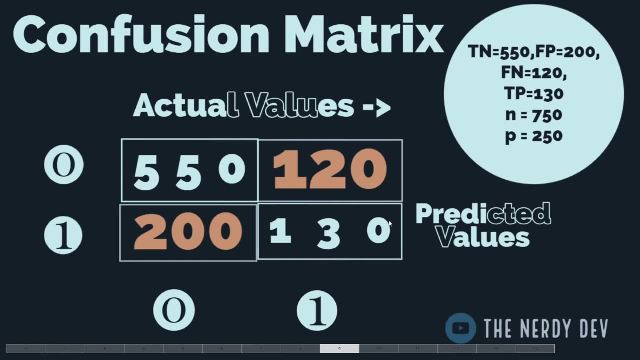 upon the number of actual negatives, which is tn divided by n. and then we have false negative rate, which is number of false negatives divided by the number of actual positives, which is fn divided by p. so now let us consider an example and compute all the above terms by assuming a test data set. 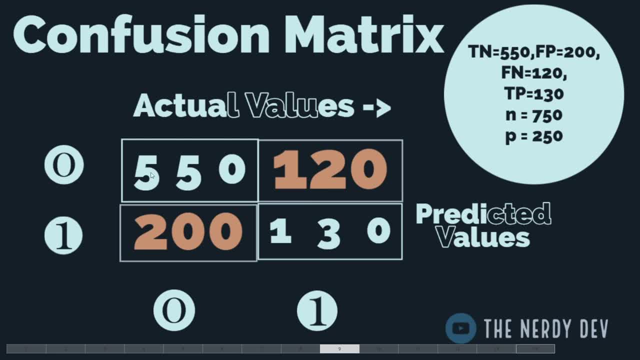 that has 750 negative points denoting class zero. so if you total this up 550 plus 200, it comes out as 750, which is 750 negative points denoting class zero, and 250 data points denoting class one, which is 120 plus 130. so now we know that each cell of the matrix represents. so now we know what each cell 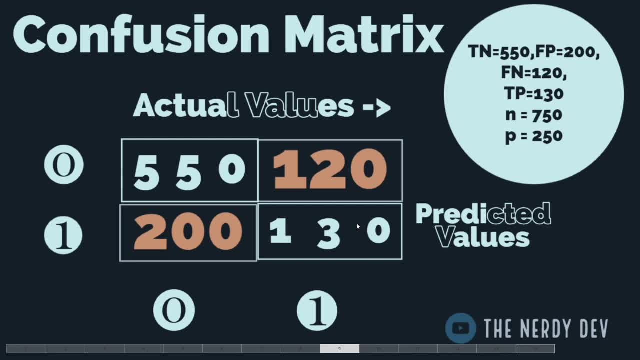 of the matrix represents. let us fill some values within each cell. so if we take on the values for which is true negatives as 550, the false positives as 200, the false negative as 120 and true positive as 130, so you can see the total number of actual positives is 250, which is 120 plus 130. it represents 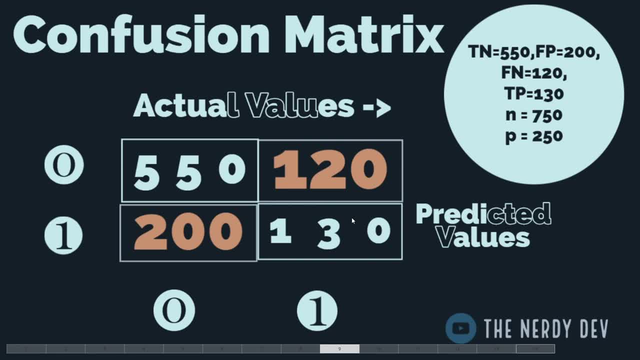 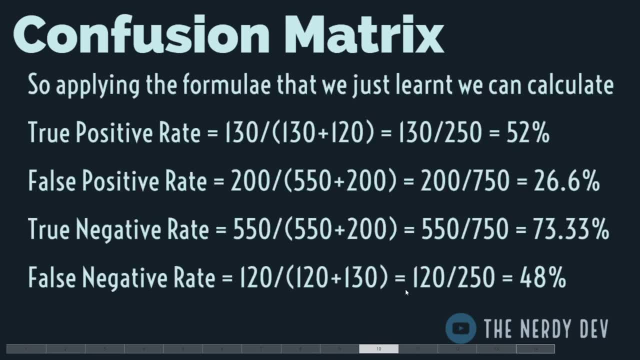 your small p, which is the number of actual positives, and the total number of actual negatives is 750, which is 550 plus 200. so if we apply the formulae that we just learned, we can calculate the true positive rate as 130 divided by 130 plus 120, which gives us a ratio. 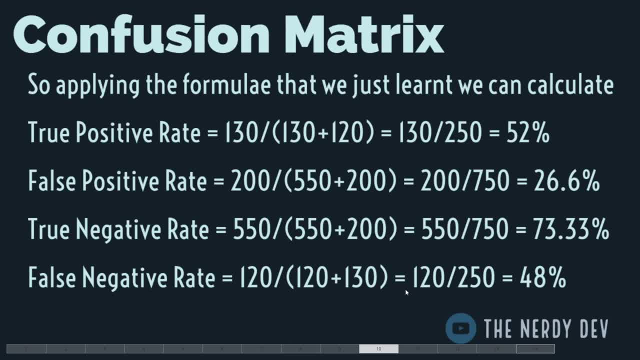 130 by 250, which can be reduced into percentage as 52 percent, the false positive rate comes out to be 26.6 percent. true negative rate is 73.33 percent and false negative rate is 48 percent. so this was all about the confusion matrix that i wanted to discuss in this video. so now let us move forward and 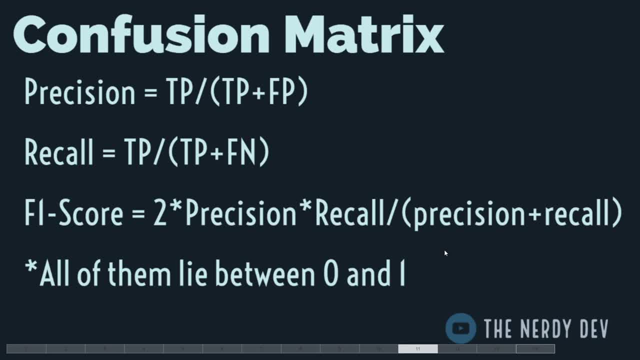 understand about the concept of precision, recall and something called as the f1 score. so these two terms, precision and recall, are very much related to confusion, matrix. so let us understand these terms now. precision says so. let us go back to the diagram. so precision says from all the points that 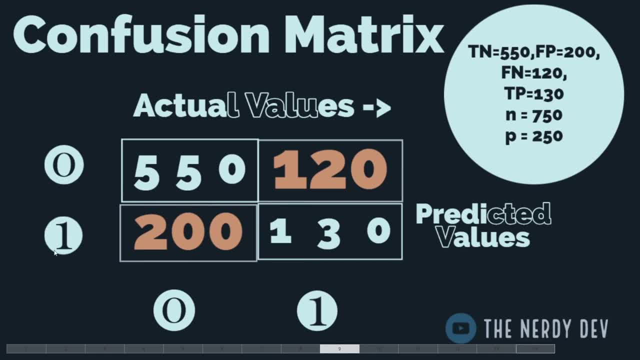 a model predicted to be positive, which is this: along this axis, which is two hundred and one third. so this row it says, for all the points that a model predicted to be positive, how much percentage of those points are actually positive. okay, so it will be 130 upon 200 plus 130, so you can easily. 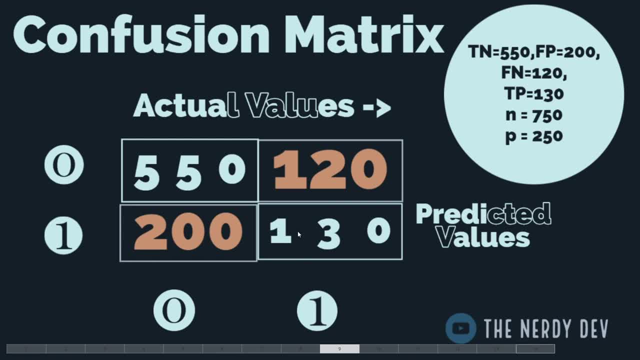 evaluate, it will come out to be some percentage value, so it will be 130 upon 330 into 100, so you can calculate the percentage for it. or you can reduce the percentage of the percentage of the data fraction, and it should lie between zero and one. so this is precision. that means 130 points. 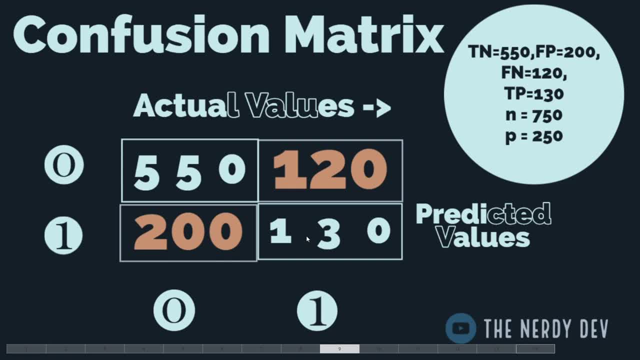 are actually positive from a collection of points that the model predicted to be positive. so this ratio is, of course, 130 upon 200 plus 130, which is 130 by 330, or you can say precision is tp, because this cell represents tp. if i go back to my slides, tp upon tp plus fp. so this is: 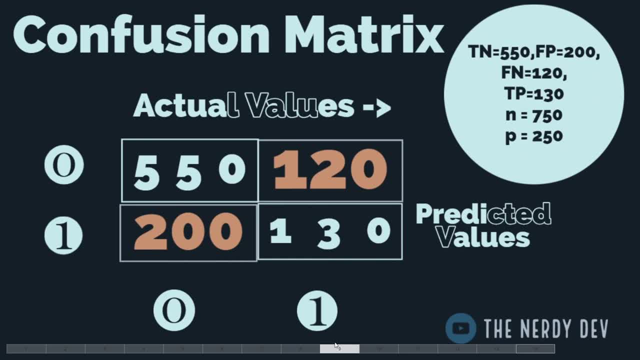 precision if i talk about recall. recall is defined as of all the points which are actual positives. that is along this direction, which is the second column. so just focus on the second column. it is defined as of all the points which are actual positives. that is the second column. how much? 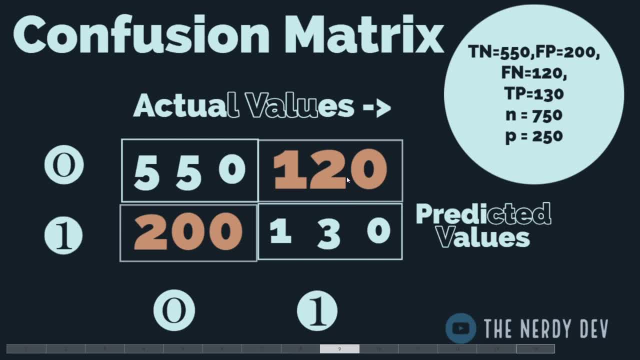 percentage of those points are also predicted by the model to be actual positive, which is 130 upon 130 plus 120. so there are 130 search points that are predicted by the model to be actually positive from a collection of points which are actual positives, that is, from 250 search points. 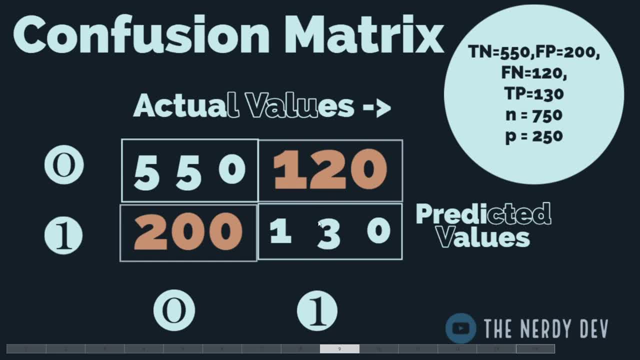 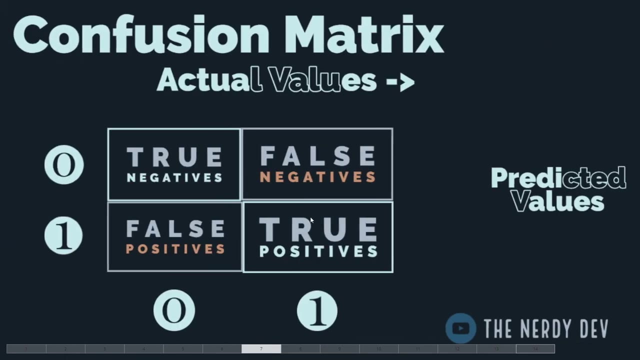 we have 130 search points that are predicted by the model to be actually positive and here the collection of points that you are taking into account are actually positives. okay, as you can see, so recall, can also be said as true positives. okay, positives upon the number of actual positives. so, if i go back to my slide seven, it is true. 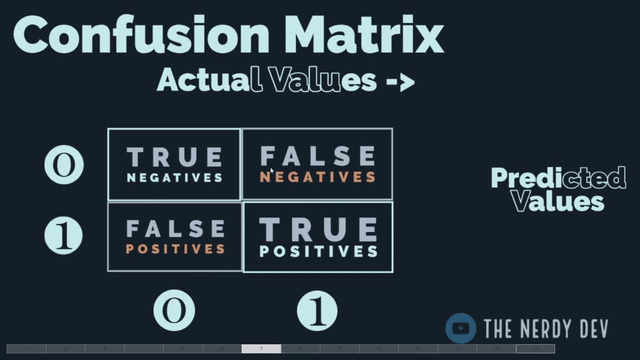 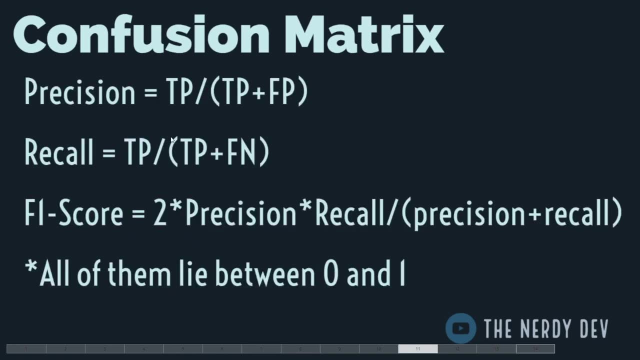 positives upon true positives plus false negatives. or you can say dp, which is true positives divided by p, and p is false negatives plus true positives. and here are the formulas. you can take a note of this. so now comes another metric which combines both the precision and recall, and that is known. 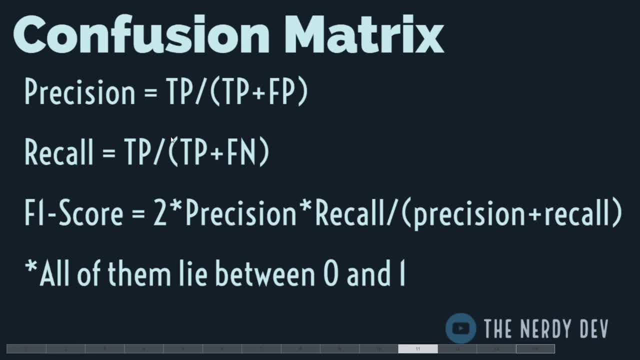 as the f1 score. remember that we want both precision and recall to have high values and they both lie between zero and one. so mathematically the f1 score can be defined as two into precision, into recall, divided by precision plus recall. so f1 score is the harmonic mean of precision and recall.